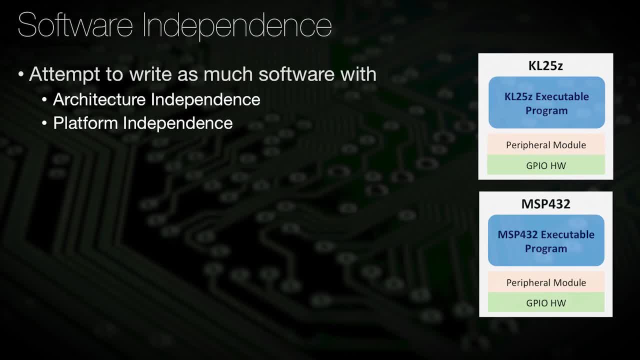 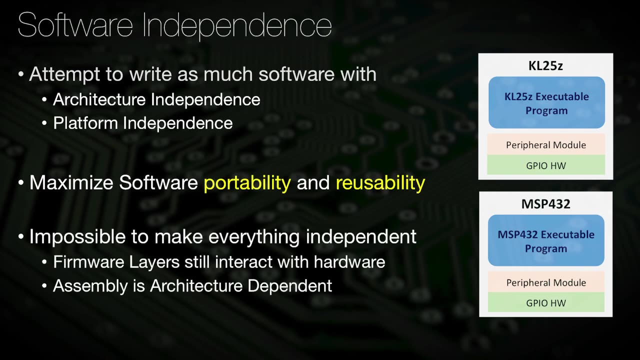 It is important as a software engineer that you attempt to develop code to be architecture-independent as much as possible. This is because it allows us to have portable and reusable code for other platforms and architectures Just by using C programming for our embedded applications. it does not mean that we have architecture-independent code. 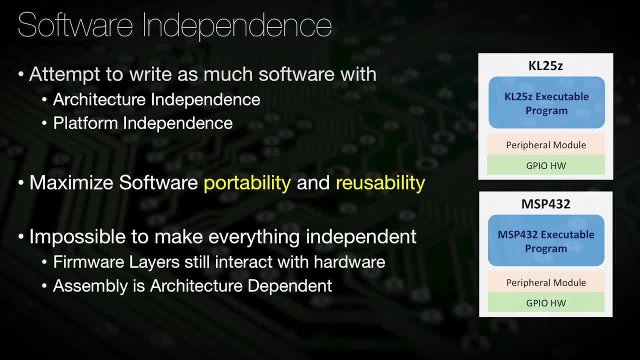 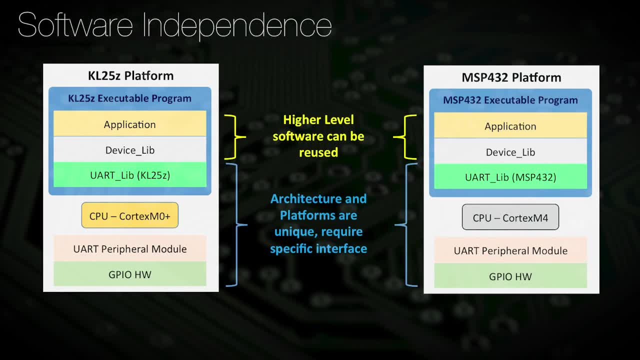 It is nearly impossible to write an architecture-independent microcontroller program. In fact, embedded systems really require the software designer to know as much about the architecture and platform as possible. This allows us to optimize our designs, utilize certain features or hardware elements in an application. 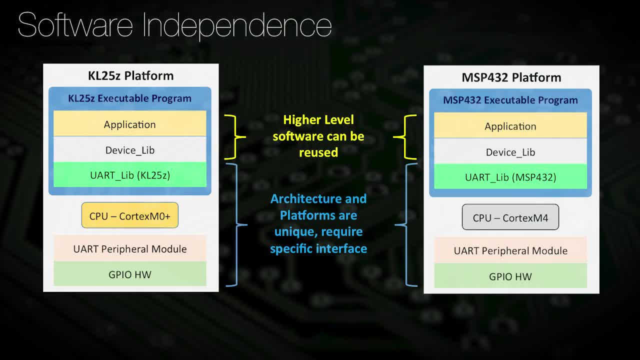 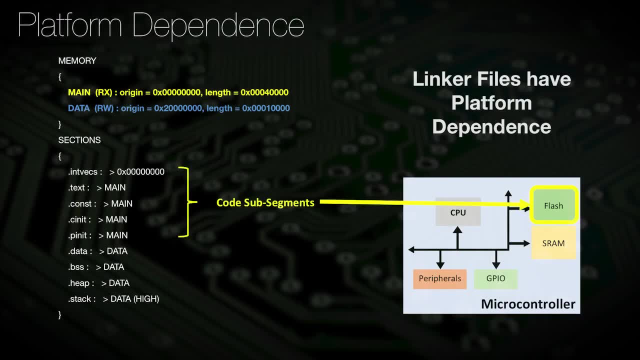 and create portability between different platforms. We discussed some basic high-level software that has platform dependencies, like the linker file with the program code and program data. The way that a compiler allocates program code and data memory is highly architecture-dependent, as there are certain specifications that map the C programming constructs to the physical memory. 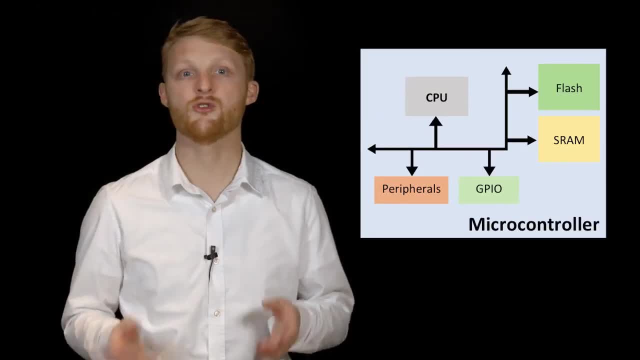 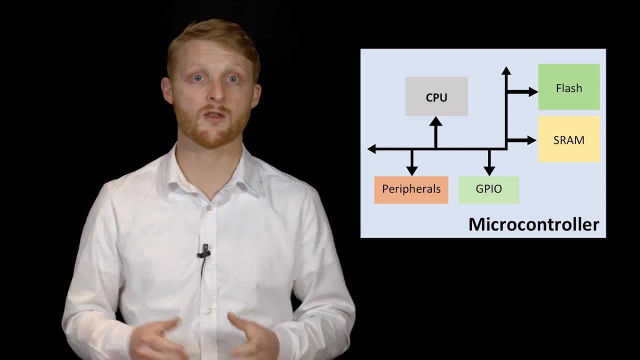 more than ever before. How does your code and your data get oriented in memory? How does your code and data get moved between the CPU and the memory interface? These are barely introduced, but they have some serious implications on your program efficiency. There are many more architecture-specific concepts an embedded software engineer needs to know about. 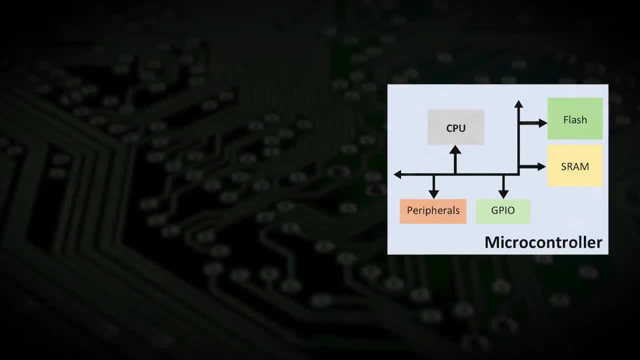 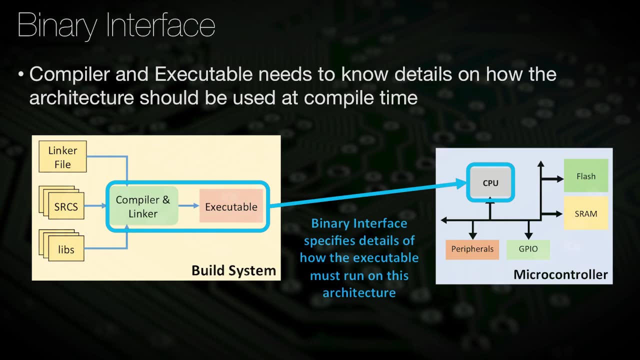 more than just this memory interaction and allocation. In addition to the engineer, your compiler must adhere to these same specifications in order to compile and install a statically linked executable into a platform. These specifications are referred to as an application binary interface or, in the case of an embedded system, an embedded application binary interface. 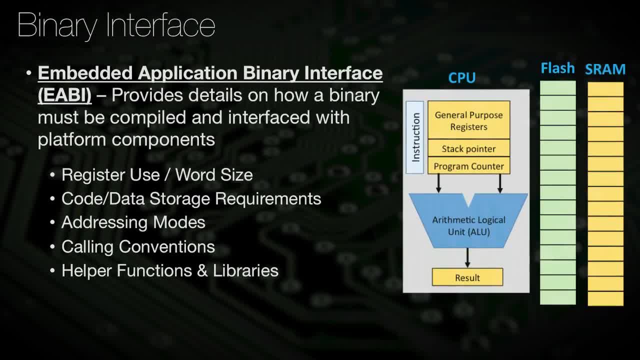 or E-A-B-I. An E-A-B-I is the specification that will provide us the details on the interoperability of our program with other statically linked programs and the underlying architecture. Let us highlight some of the basic E-A-B-I specifications you might read about. 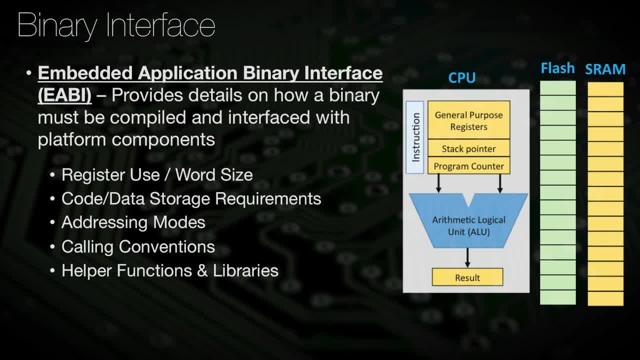 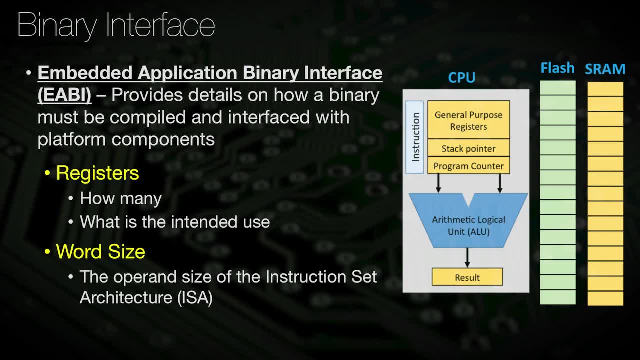 First and foremost, the E-A-B-I will specify information on how your program must be compiled. The translation of high-level to low-level language has specific requirements on things like register use and word size. The word size is the operand size. the instruction set architecture was defined around. 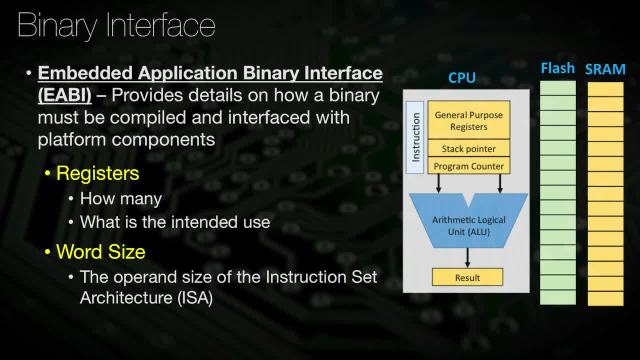 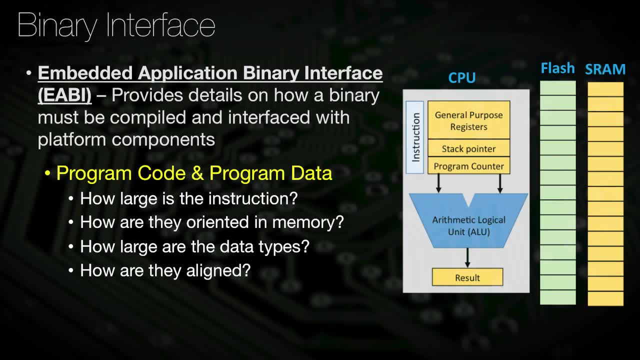 All operations are written to perform actions on data of this size most optimally. There are specifications on how program code and data are physically sized and placed into memory. The C programming language does provide us with data types, but unfortunately these are not necessarily portable. 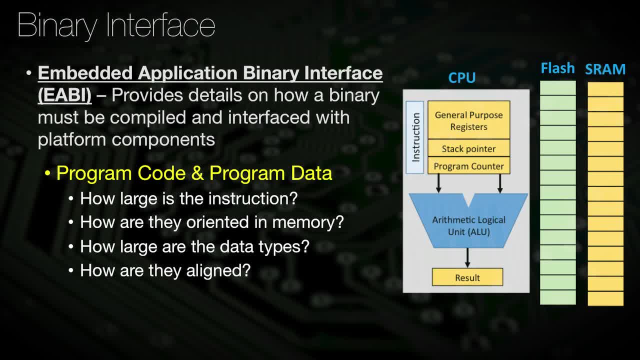 Some data types have varying size, and a compiler may even implement these types as different sizes optimized for its architecture. The C standard types are actually not the standard way developers declare data, as they can be ambiguous. Even further, allocated information will be aligned within specific boundaries with memory. 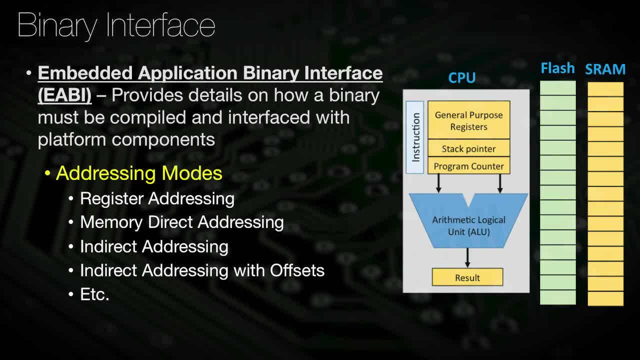 There are also addressing modes. For example, if you have a program that is running on memory, you will need to have a program that is running on memory. The C standard types will provide information on how your program operates on memory. This specifies information like how your program reads and writes program data. 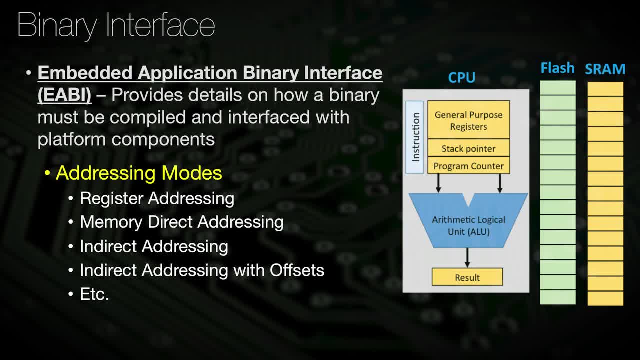 The assembly instructions need to know where that data is and the best way to access it. In addition, the compiled segments that we discussed regarding a linker file and the outputs of building are also specified in an E-A-B-I. The calling conventions we discussed briefly with the stack memory segment. 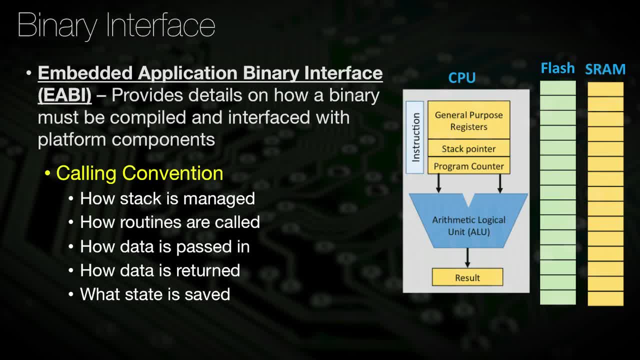 are specified in the E-A-B-I as well. It will provide responsibilities on what needs to be saved or restored by the calling routine and what needs to be done by the routine being called. This process is directly related to the implementations of the stack and the CPU registers. 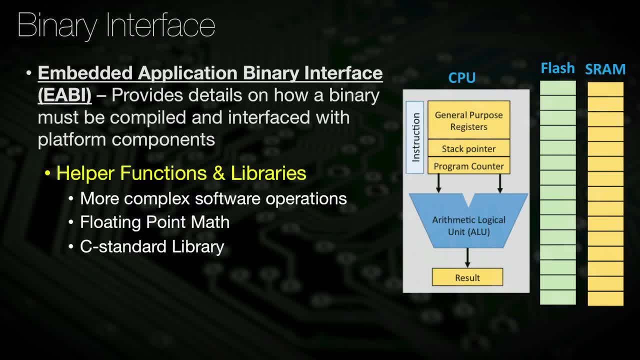 Finally, the E-A-B-I will also specify which libraries or helper software functions that perform more difficult software algorithms that you can write and see but not necessarily are supported by an architecture. Hardware without floating point support must implement all floating point math with software routines. 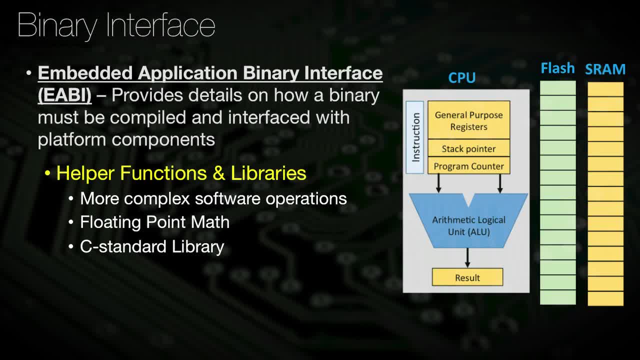 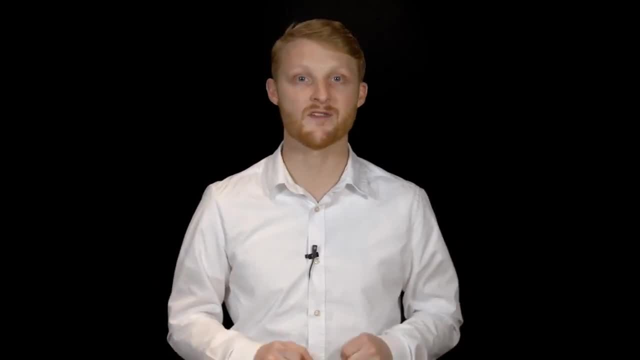 If there are existing statically linked libraries, like the C standard library, this will also specify how executables need to interact with the standard library. All of these examples were just basic introductions into some architecture requirements that the compiler handles behind the scenes. Developers need to know these too, as some serious bugs can be introduced.